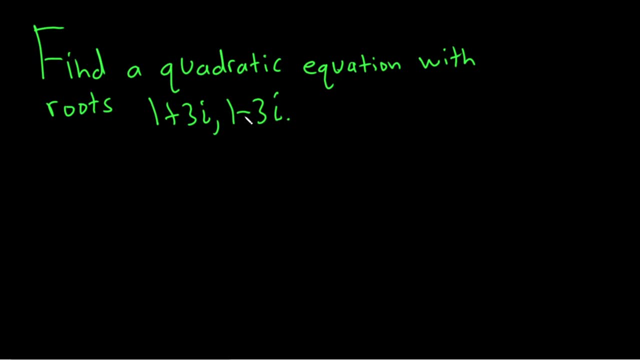 Hello, In this problem we're going to find a quadratic equation with these roots. Let's go ahead and work through it. Solution. So there's a couple of different ways of doing this problem, So let's try to do this a very short way. 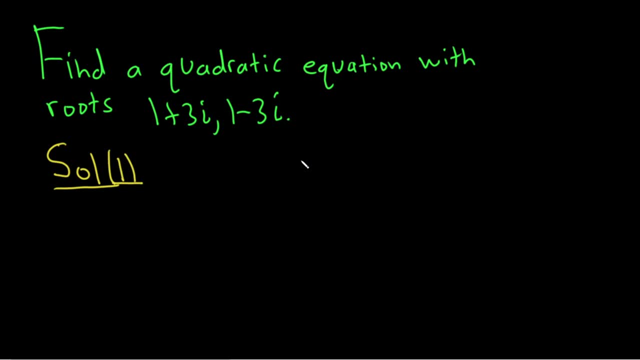 So I'll show you two ways to do it. So solution one. So solution one is going to require, or it'll be helpful if we simplify these roots. In theory, the roots here are 1 plus or minus 3i. 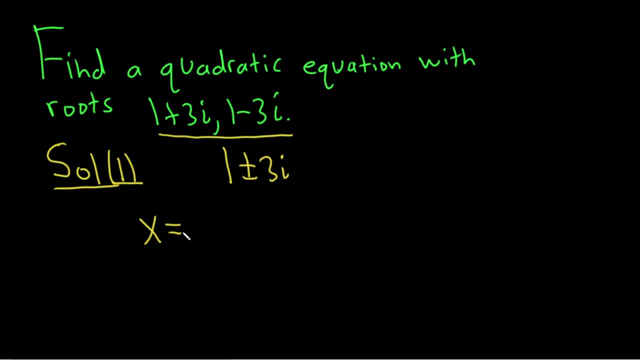 So we can say that x, the roots, are equal to 1 plus or minus 3i, And from this equation we can construct a quadratic equation in x. So to do that, what I'll do first is I will isolate the imaginary part by subtracting 1 from both sides. 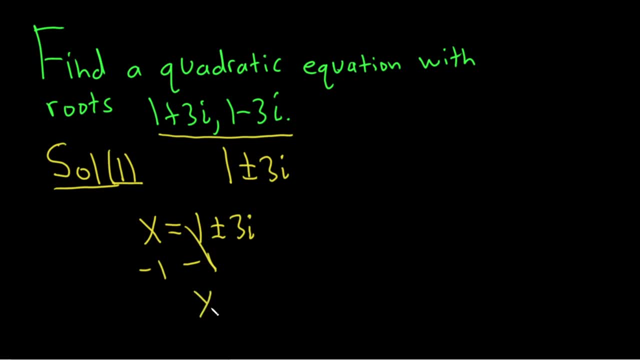 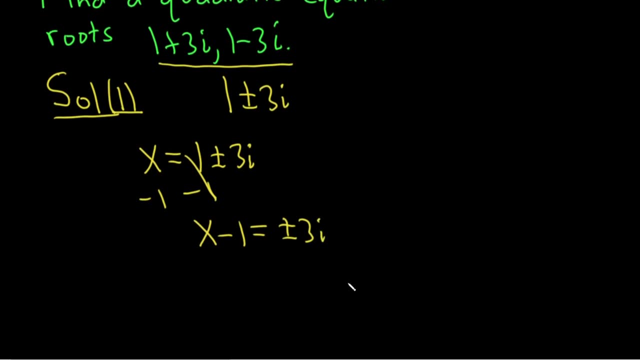 Subtract 1, subtract 1.. So we get x minus 1 equals plus or minus 3i. Now we're going to do something which might appear dangerous, but it's not. We're actually going to square both sides with the plus or minus there. 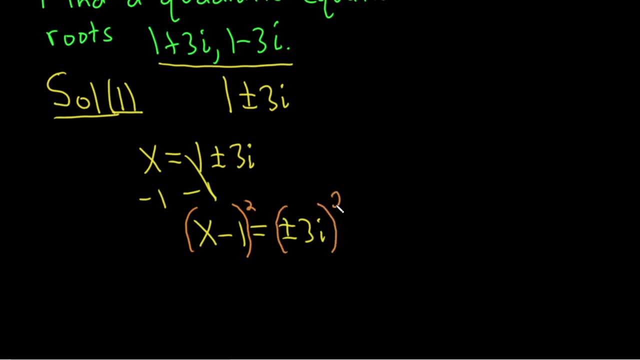 Just like this. So we'll put the parentheses around the whole thing like this: On the left-hand side we have x minus 1 quantity squared, So that's an easier one that you might know. It's x squared minus 2x plus 1.. 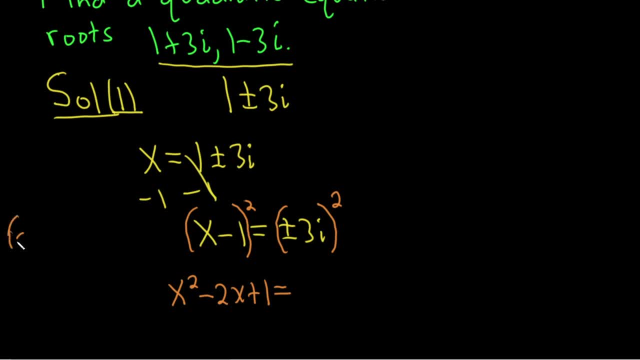 If you don't know it, it's okay, You could use this formula here: a minus b, squared. So you square the first one, so that's your a minus 2, and then you double them. So you're doubling them: 2ab plus the last one squared. 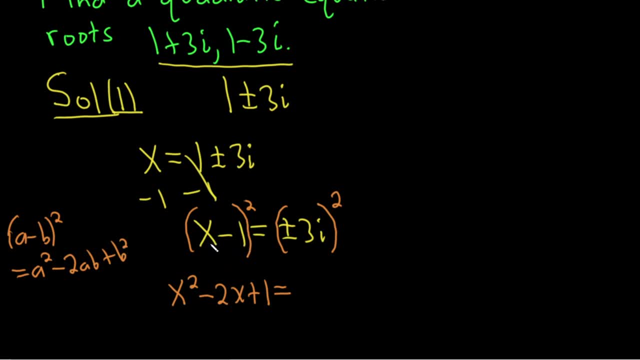 So you square the x, you multiply the negative 1 in the x, and then you multiply by 2, and then you square the last one Over here. when we square the plus, it's just going to be a plus And there's really a negative. 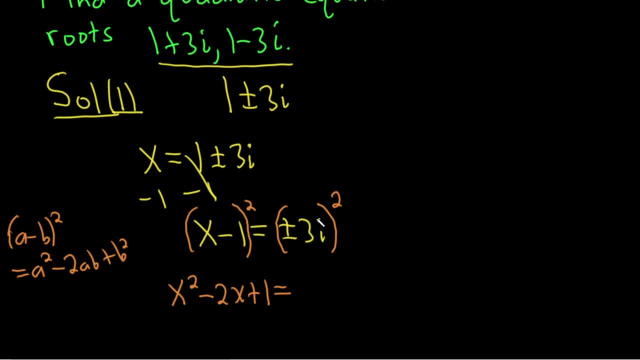 There's a negative 1 here. if it's negative 3i but the 2 here it's being squared so it goes away. So this is completely irrelevant. So you just get 9, that's 3 squared, and then i squared is negative 1.. 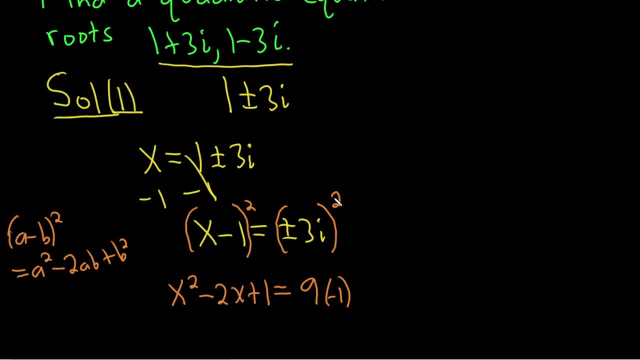 Because, again, if it's plus 3i, if it's plus 3,, 3 squared is 9.. If it's negative 3, negative 3 squared is 9.. So, in any case, the plus or minus 3 is going to be 9.. 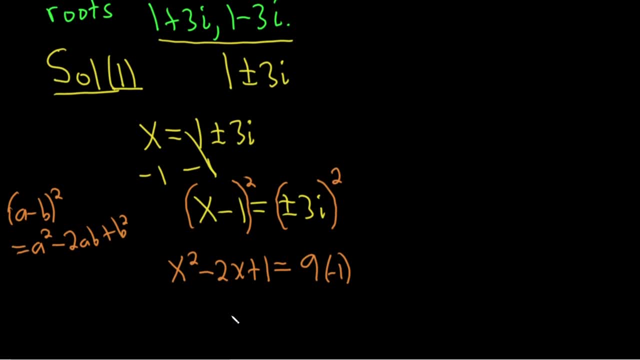 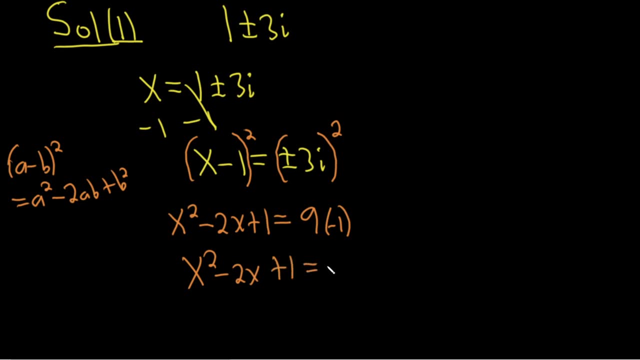 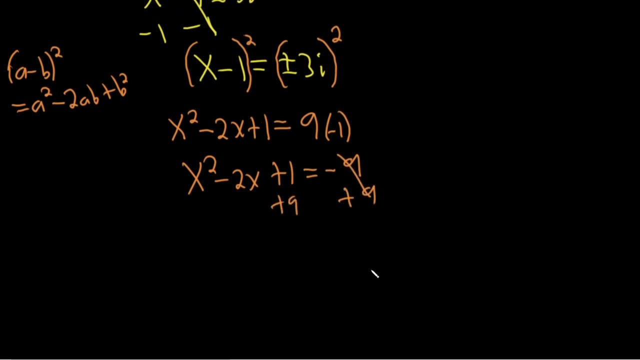 And then i squared is negative 1.. This is now x squared. x squared minus 2x plus 1 equals negative 9.. And so now you can add 9 to both sides. so plus 9, plus 9.. And so we get: x squared minus 2x plus 10 equals 0.. 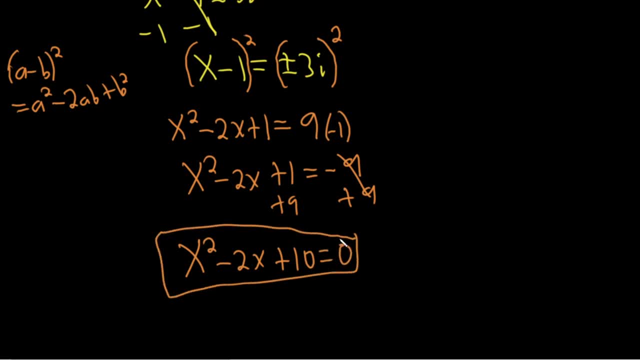 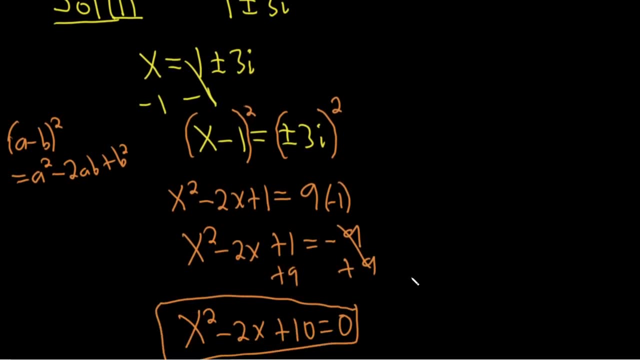 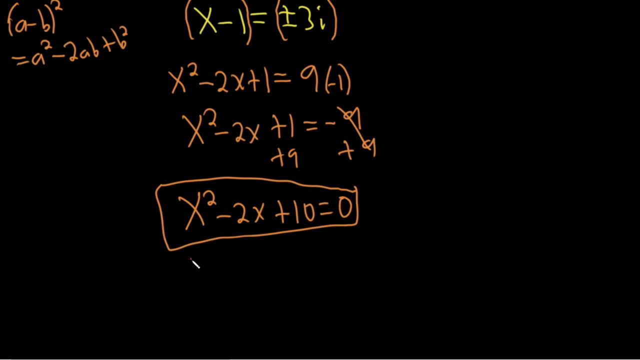 And that would be the quadratic equation. By the way, if you look at the original question, it did say: find a quadratic equation with roots. The reason it said a is because there's infinitely, infinitely many solutions. right? If you wanted to be silly, you could just take the number 3 and multiply it through. 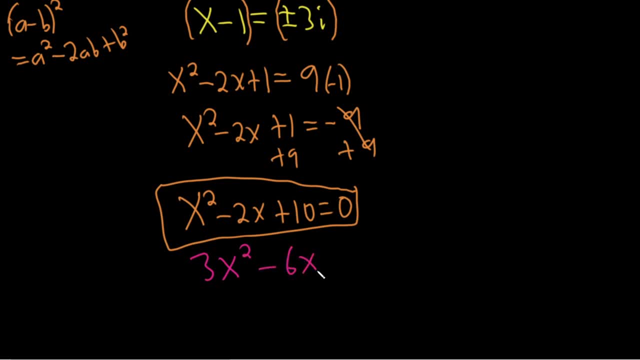 Another possible answer would be: 3x squared minus 6x plus 30 equals 0, right. The solution is certainly not unique. This is also another acceptable answer. But nobody does this right. Why would you? But it's important to be aware of stuff like that because it does come up in different. 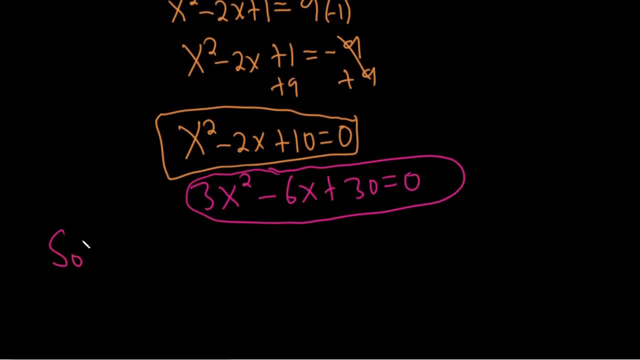 situations: Okay. another solution, which is a little bit longer, is to realize: okay, we have a solution. Okay, we have a solution. Okay. another solution, which is a little bit longer, is to realize: okay, we have a solution. 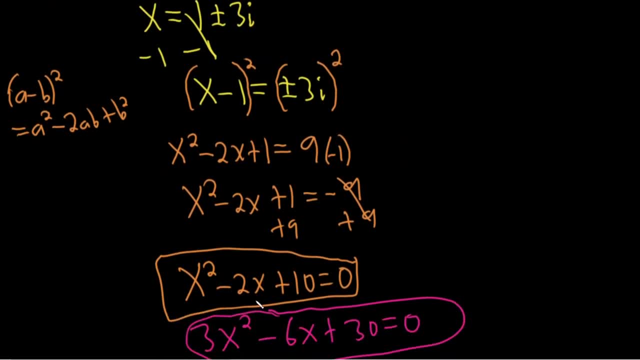 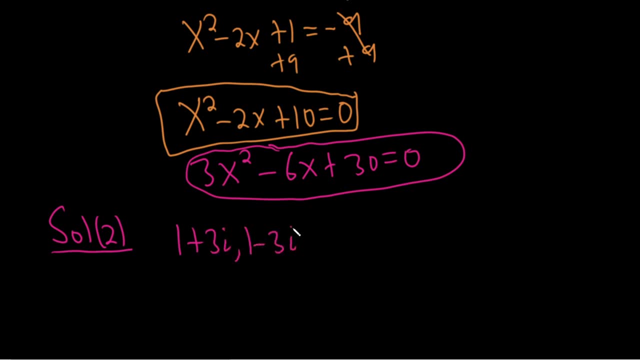 We have a solution. These are our roots. But we know that if 1 plus 3i is a root, then a factor of our equation must be 1 minus 1 plus 3i. That's going to be one of the factors of our quadratic equation. 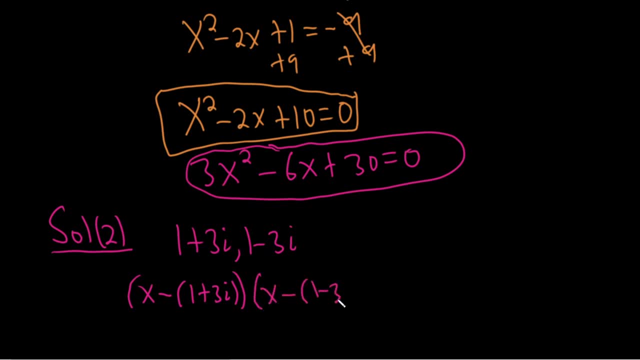 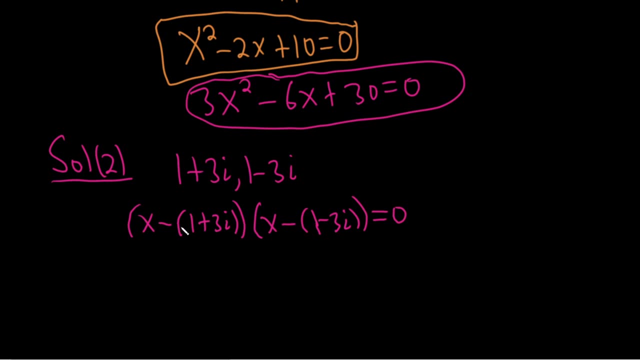 And the other factor is x minus. Notice the ultracareful, Ultra careful placement of the parentheses, right. It's really important that they're around the entire root of the equation. So again, in general, if c is a root of an equation, then x minus c is a factor for polynomials. 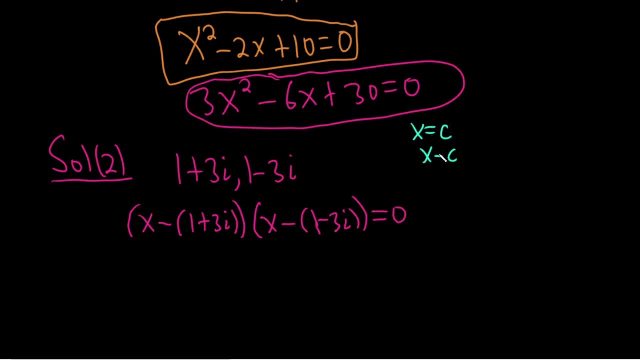 So, for a quadratic equation, if c is one of your roots, x minus c is a factor. So we have x minus c, x minus c. Okay, let's go ahead and carefully distribute the negative 1, right, There's an invisible negative 1 here and here. 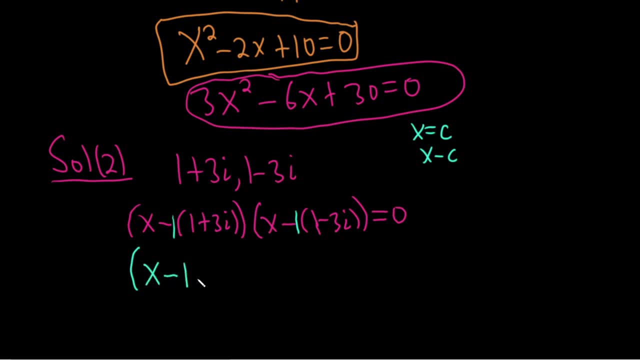 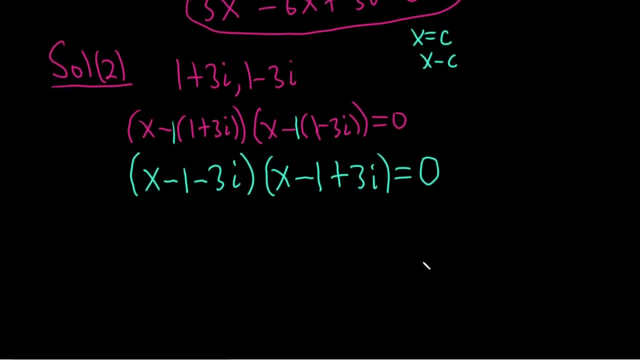 So this will now be x minus 1 minus 3i, And this is x minus 1, and then this will be plus, because it's negative 1 times negative 3i. Okay, so now watch this. Now, what we can do is we can put a parentheses here. 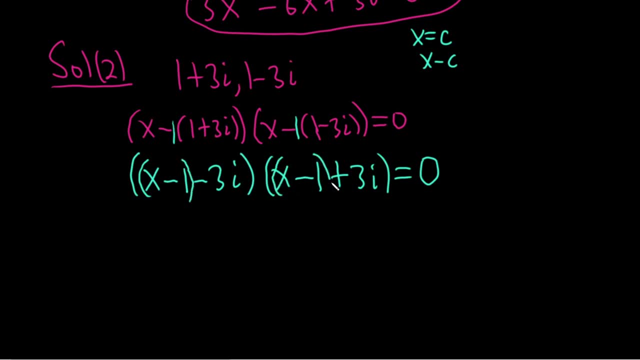 This is super clever And put a parentheses here. Okay, and then now we're going to use a super powerful formula. If you have a minus bi times a plus bi, that's the same thing as a squared plus b squared. So here it'll be a squared which is x minus 1, squared plus 3 squared, which is 9.. 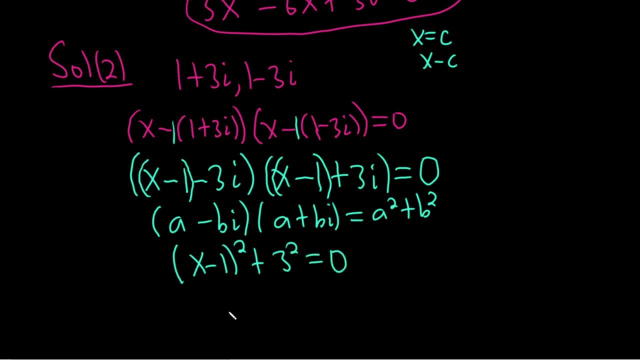 So I'll just put 3 squared As before. we know that x minus 1, quantity squared, is x squared minus 2x Plus 1, and then we have 3 squared, which is 9.. And so this leads to x squared minus 2x plus 10, and that is equal to 0.. 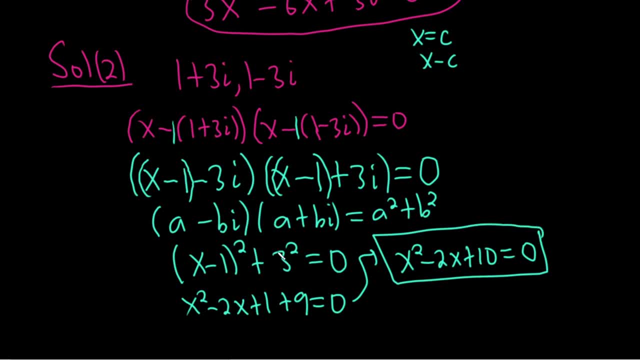 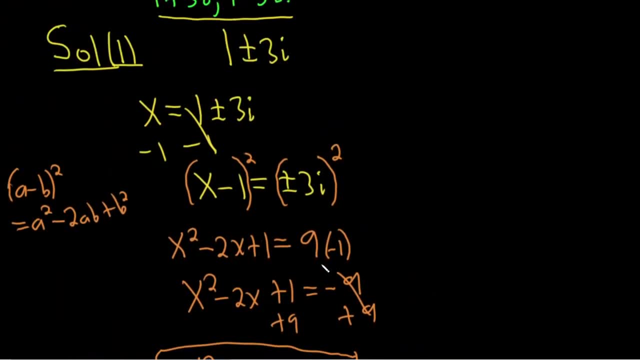 And that would be it. right? That would be the quadratic equation. So which one is easier? I'd be interested in knowing what you think. I personally think the first solution is much cooler. I used to always do these problems this way. 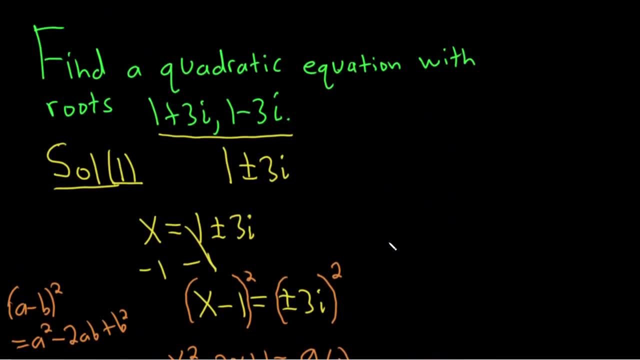 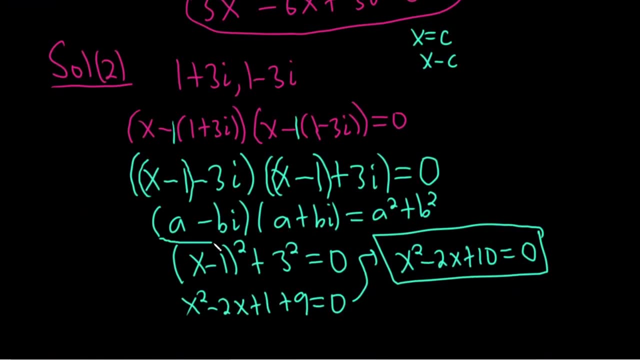 And then one day I thought- or someone showed me this- I thought: oh, that's really clever. So a little bit cleaner, right, A lot less work. This is certainly a lot more work. It requires that you know this formula. 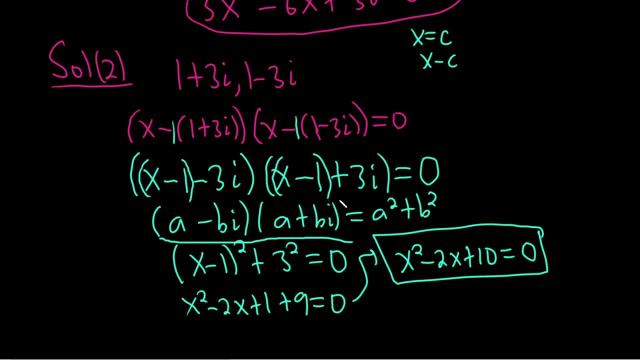 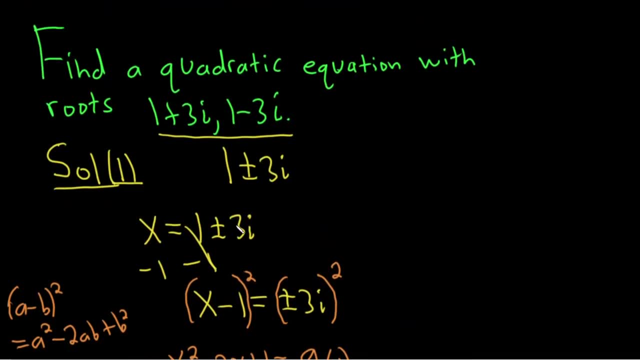 You could foil this, but it would be not fun. Also, you have to be extra careful here with the parentheses. It's just more work in general. This is a lot more to the point. I hope this video has been helpful. Good luck. 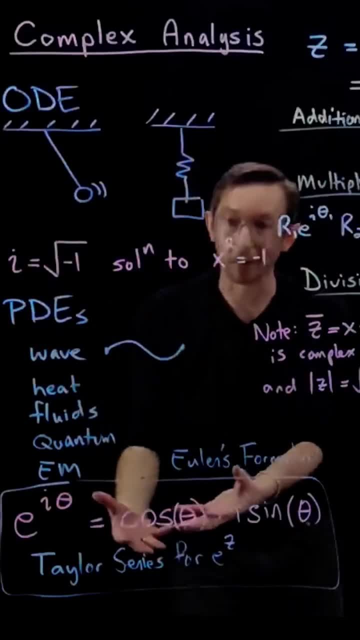 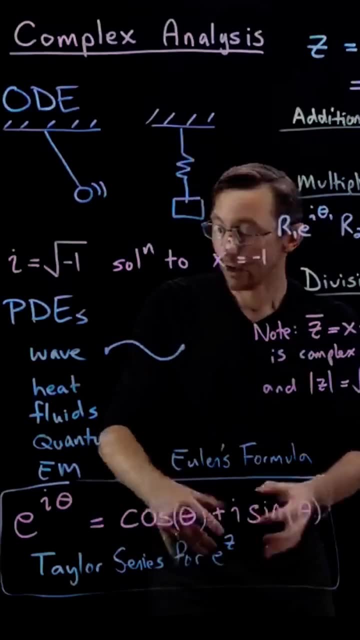 Equations and partial differential equations, just like I showed you down here. It's going to be very, very natural sometimes to think about- Instead of writing things in real plus imaginary part, just to think about it in terms of, you know, This kind of polar form e to the i theta. that's going to be more useful when we think about the wave equation, when we think 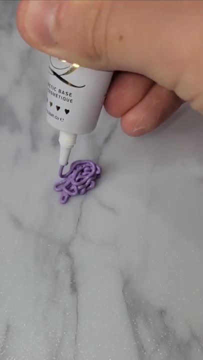 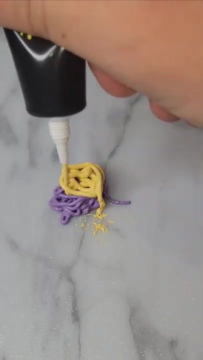 I would say that understanding color theory when it comes to anything related to makeup is something that's super important for people to understand. So right now, i'm going to take a purple and a yellow product and i'm going to combine them together Because on the color wheel, purple and yellow are across from each other.